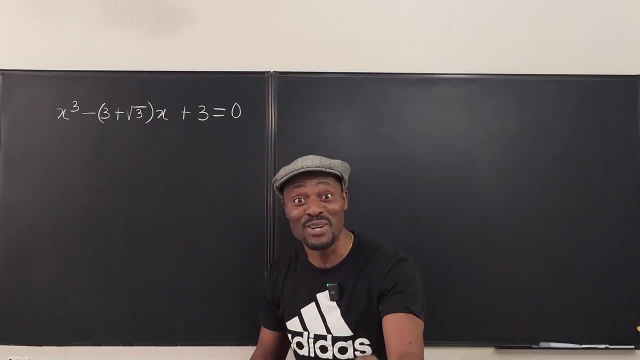 you're not thinking of what to do. but as soon as you think of what to do and you apply it, it just becomes so easy. and that was what happened. I kept thinking about it and ultimately I found the answer, and when I was done- guess what? I said: okay, I actually didn't think of it. 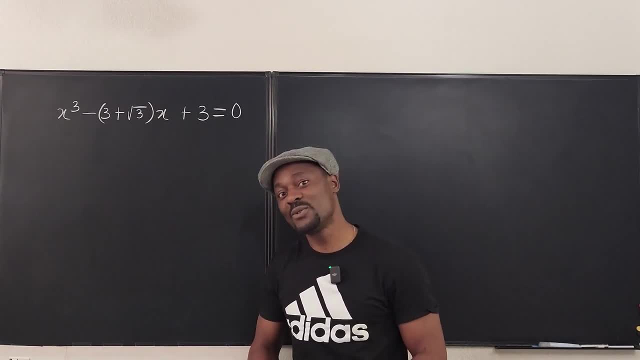 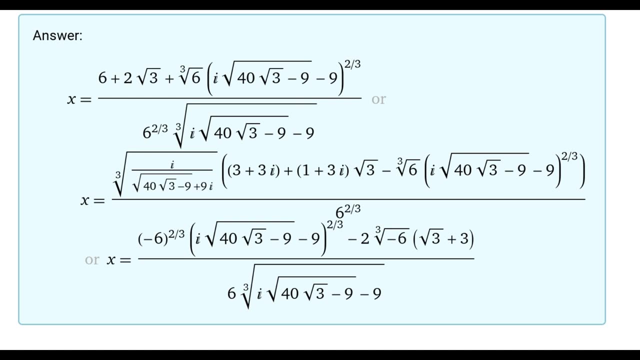 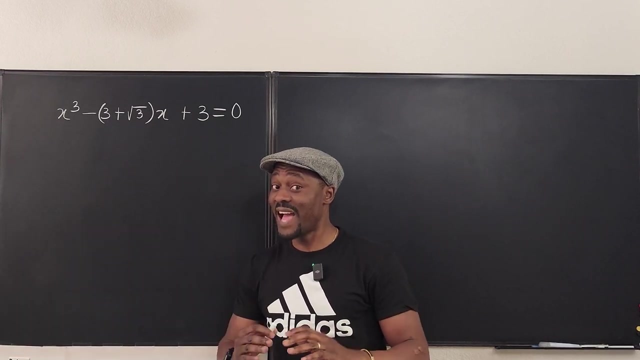 I plugged it into Woe From Alpha and this was what the answer was: Yeah. now, that was not the answer that I got, but I think the Woe From Alpha algorithm worked it out that way and that cannot be the answer. if it's an Olympiad problem, It has to be something that. 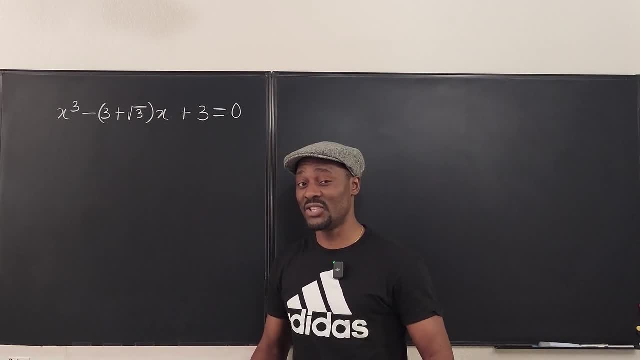 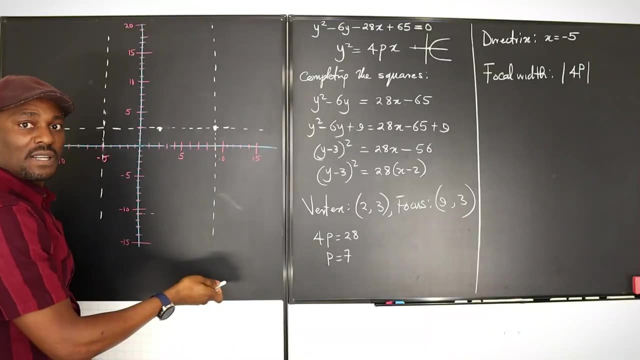 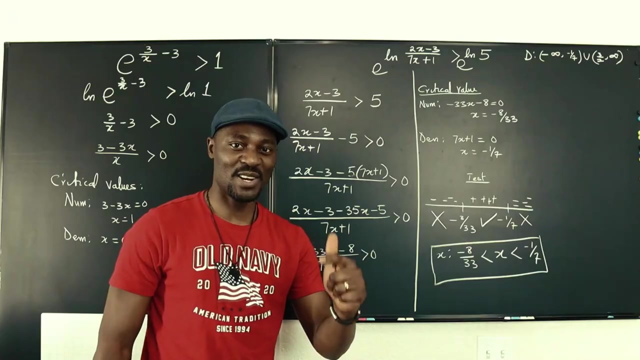 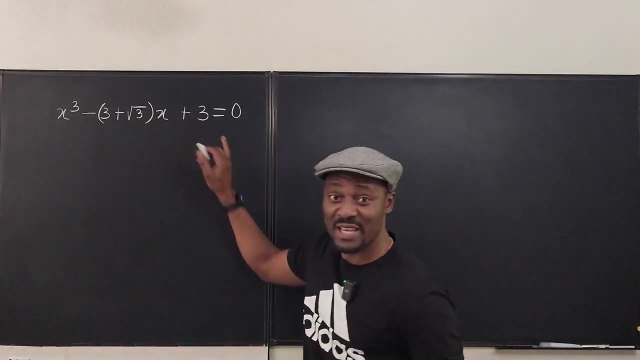 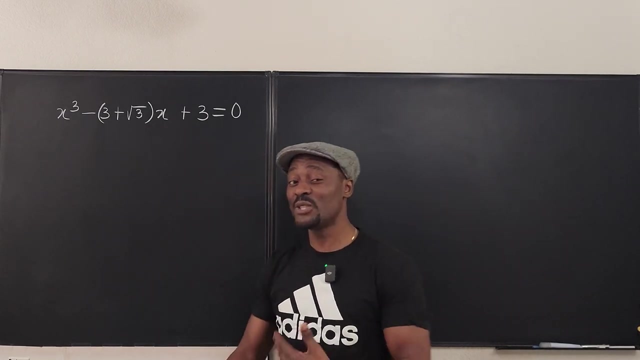 is easy to understand and what I have as answer is easy to understand and I'm going to show you. Let's get into the video. The very first thing I decided when I saw the problem is that, because it is a cubic equation, it must have three solutions. I always tell myself that. and if it must have three solutions, 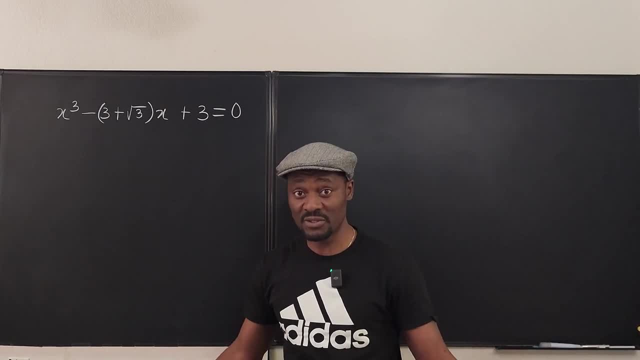 two of them may be the same or all three may be different solutions, but none of the methods that I have or that I know worked. Okay, I couldn't see it as a difference of two cubes. I tried to generate difference of two cubes, but it just didn't work. 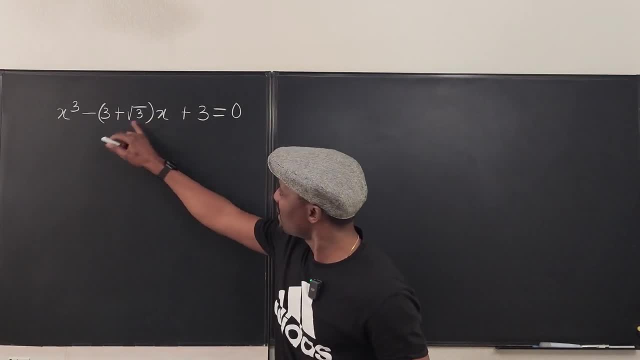 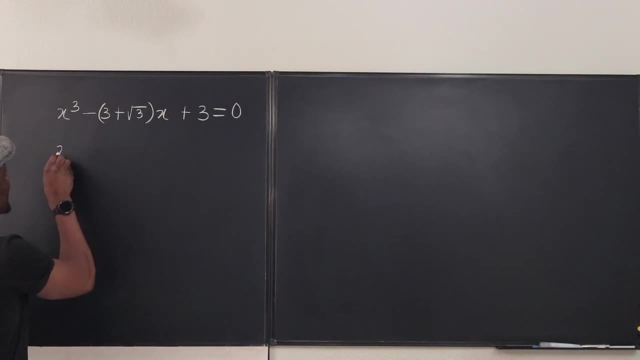 And then I said, maybe if I distribute this x, I might be able to rearrange and factor. So I did that. So this is what happened. I did x cubed minus 3x. This would be minus square root of 3x plus 3 is equal to. 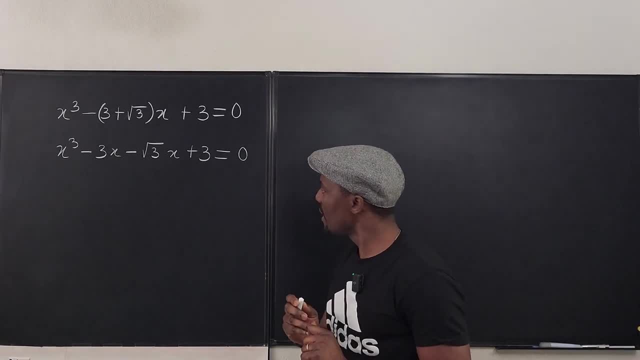 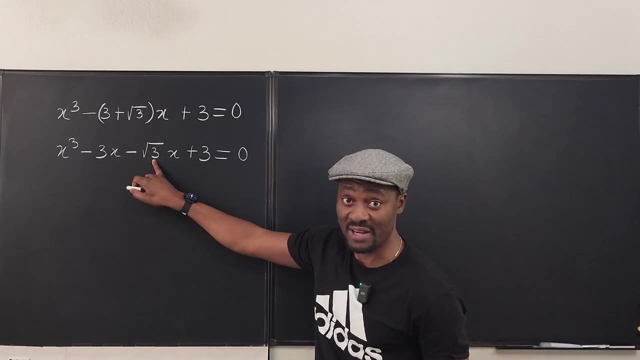 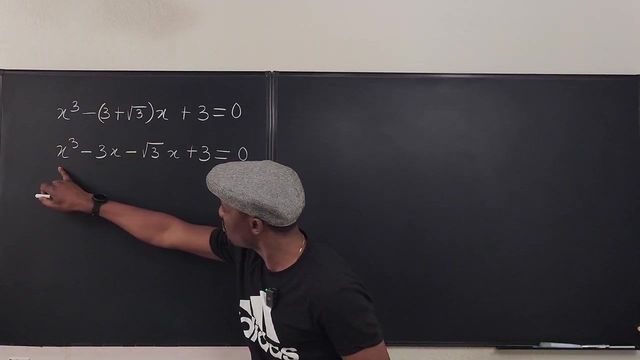 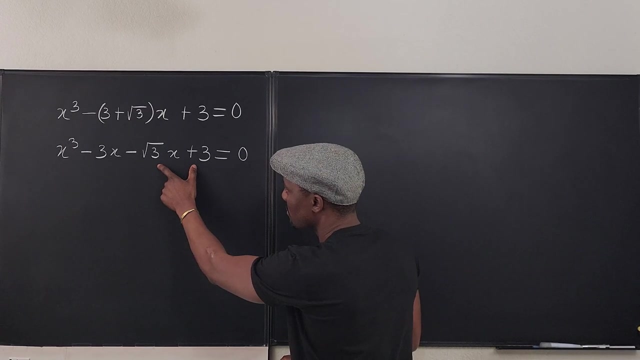 Zero. Now, if we try to find things that would go- because this is the problem, this and this are the problem that I have- actually, If I try to put this and this together, if I factor out x, I'm going to have x squared minus 3 here. But if what would I factor here? There is no x squared minus. 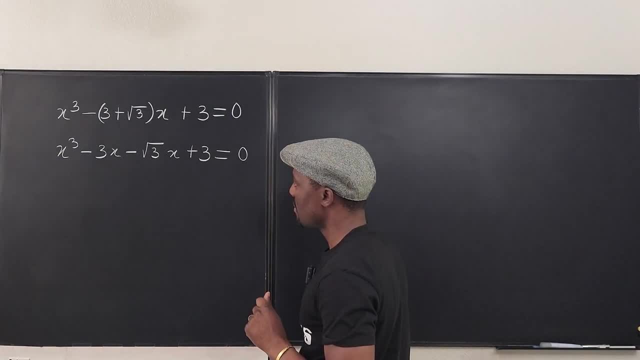 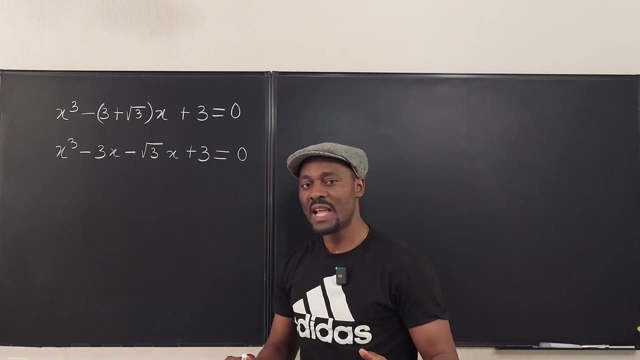 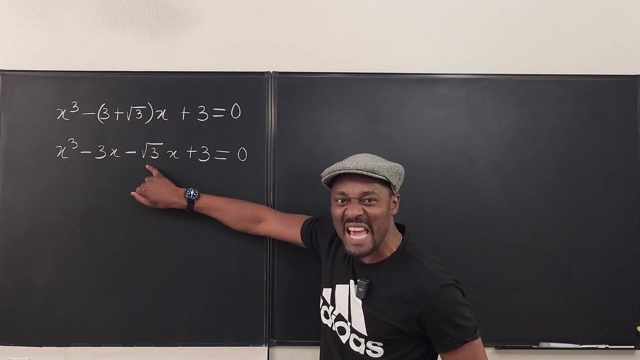 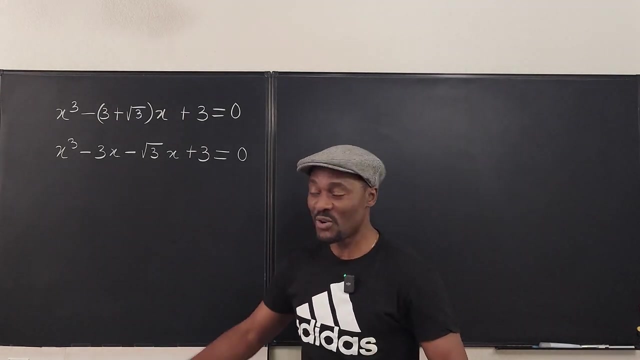 3. Yeah, and I'm not factoring out the same thing. So it's a problem. Now, and this is where I started thinking, what if this square root is the main problem? Because actually this is a problem. I don't think that you find it as a common thing to have. 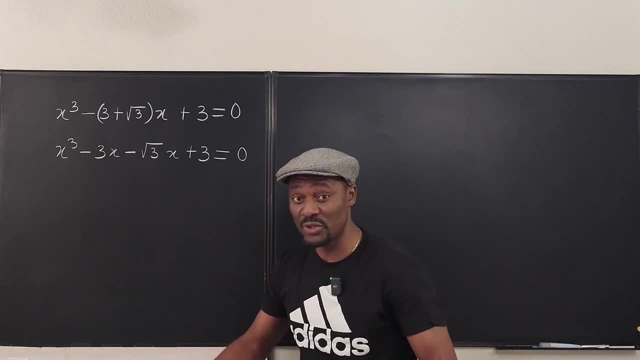 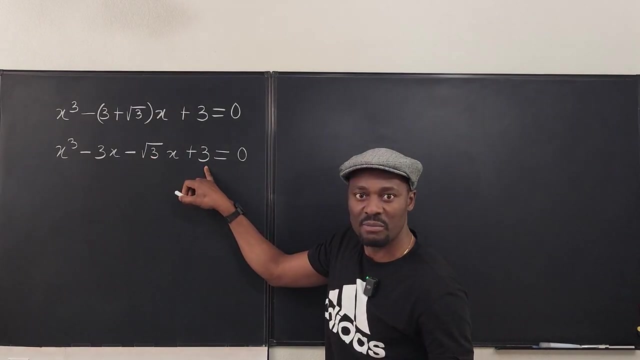 the coefficient of x being irrational. Most of the equations we solve are rational, and then our answers may be irrational. So I said, what if I treat this as another variable and this is the square of this variable? Can I do so? Is it easier to see something to factor? And that was when my eyes were opened. 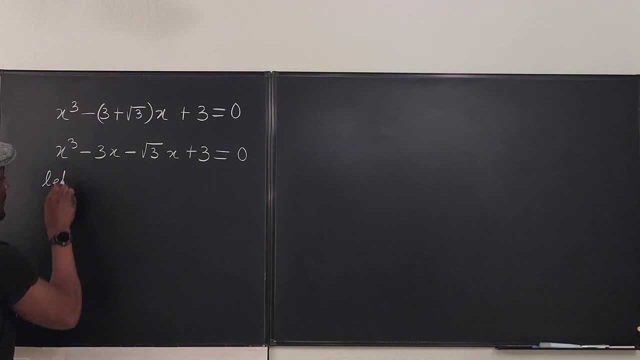 OK. so again I said: let y be equal to the square root of 3.. So watch this Now I have. this became Zero, became x, cubed minus, you see, the square root of 3, this simply means that y squared will be equal. 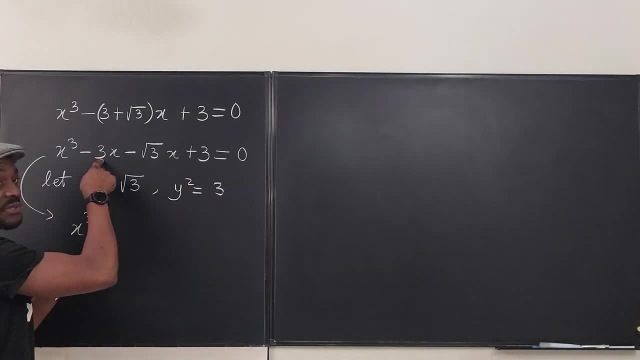 to 3 if I square both sides. So instead of writing 3, here I'm going to write y squared x, Here I'm going to write y, and here I'm going to write x plus y squared equals 0.. Now I want you to start. 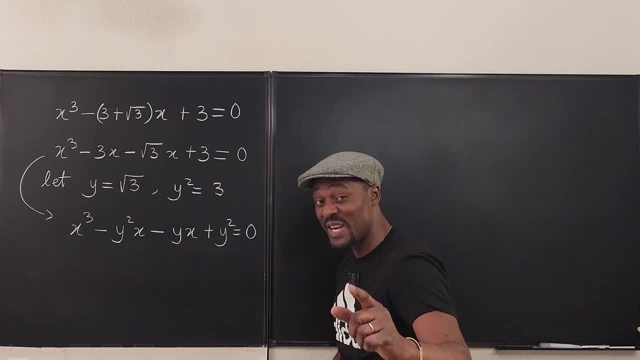 looking at things you could see. Now we need to find some kind of factoring somewhere here. You see, because we've written this as a square, it is easier for you to see difference of two squares if you take out one x from both terms. 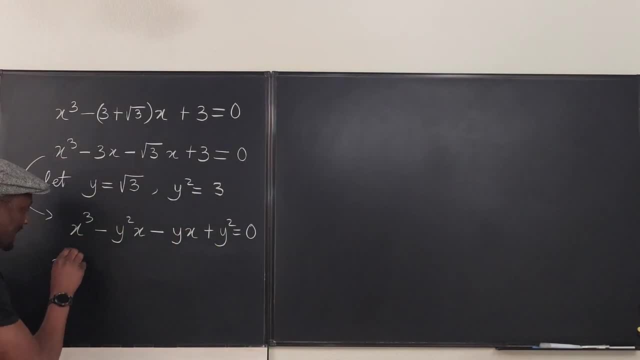 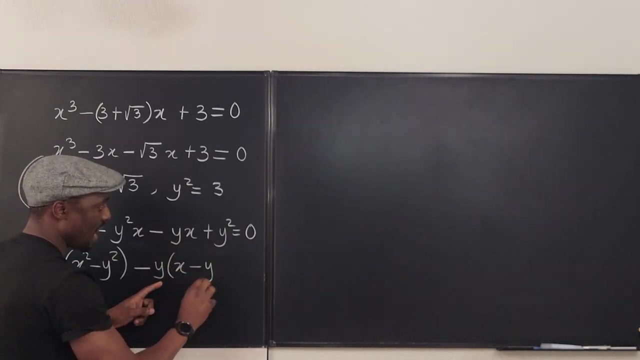 So we can see this as if I take out x, I'm going to have x squared minus y squared. What can I take out from this? I can take out negative y minus y and if I, I'm going to have x minus y remaining. 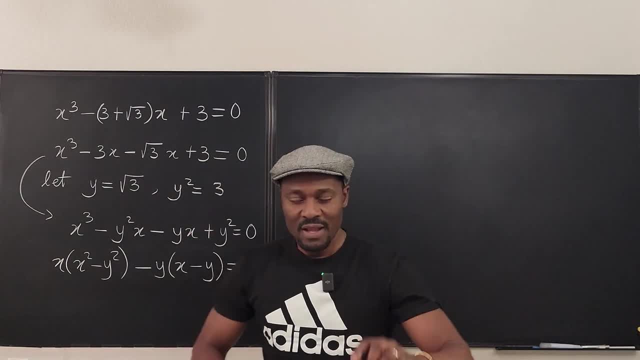 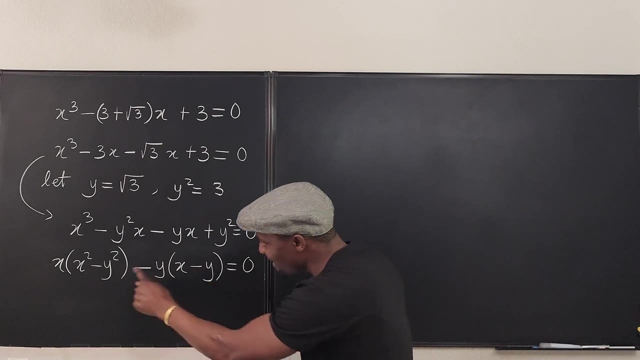 equals 0.. Now you get excited when you get this thing factored, if what is here is also what is here. But at this point this is not this. But I see this inside this, because this is the difference of two squares, that I can further break this down So that I have x times. this is difference of two. 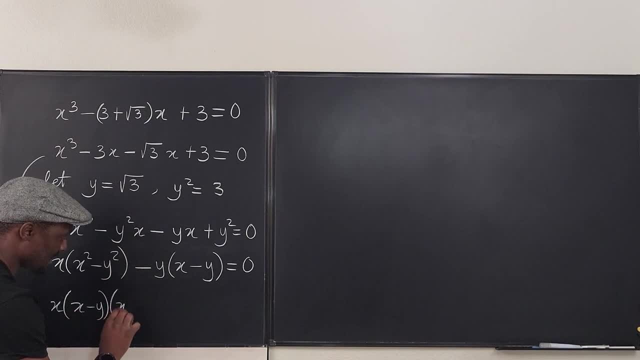 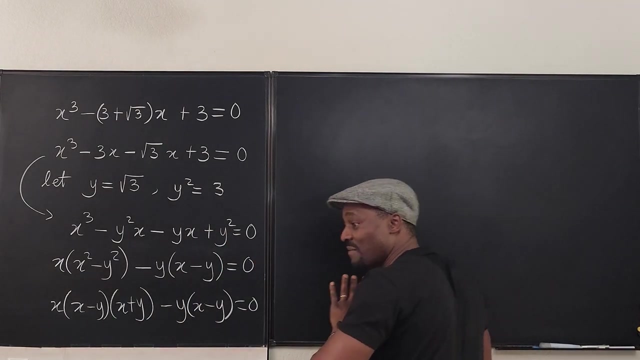 Squares x minus y, x plus y minus y times x minus y is equal to 0. That's it, it now. i see x minus y here, i see x minus y here. i can factor out one x minus y term, and this guy that gave me trouble from the beginning is gone. okay, so what we have now is, if i take this out, 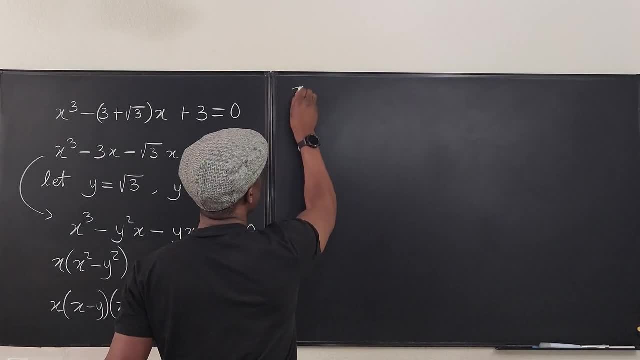 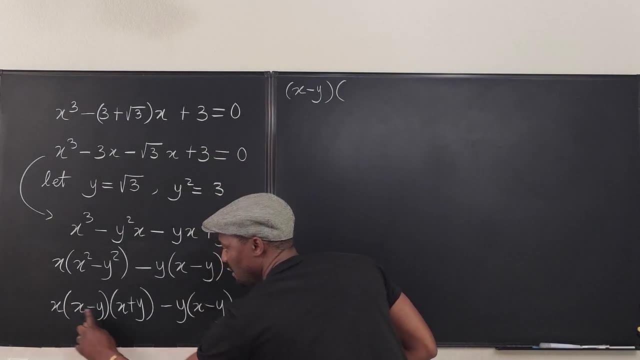 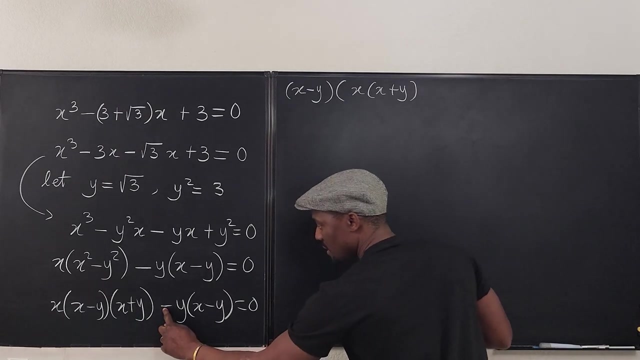 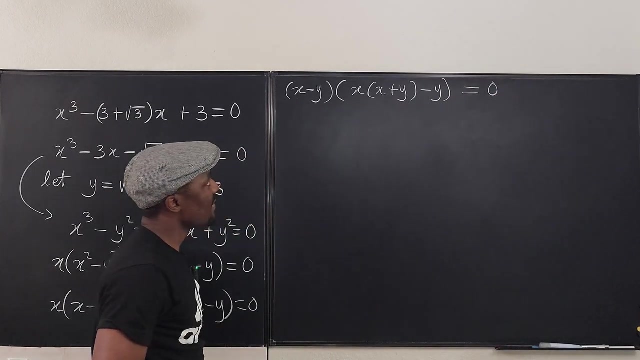 so i take one out from here, and here i'm going to end up with x minus y times what. what's going to be left? if i take this out factored, i'll have x times x plus y, x times x plus y minus. oh, there'll be y remaining minus y, and this is equal to zero. let's clean this up. so we have x. 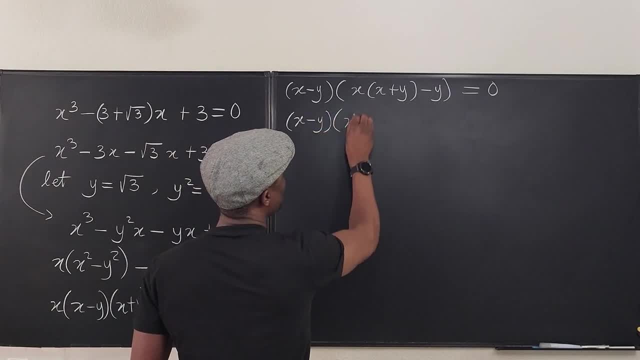 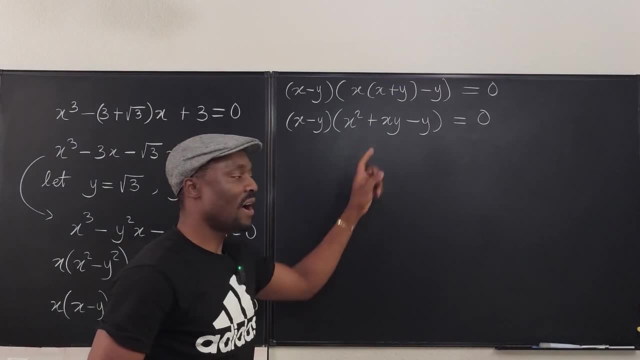 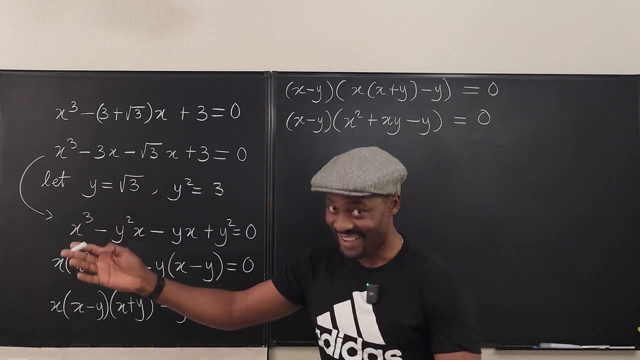 minus y times. this is x squared plus x, y minus y. is there anyone watching this video who doesn't know how to solve this? remember the assumption we made. we said: let Y be aha the square root of 3. so this is X minus the square root of 3. 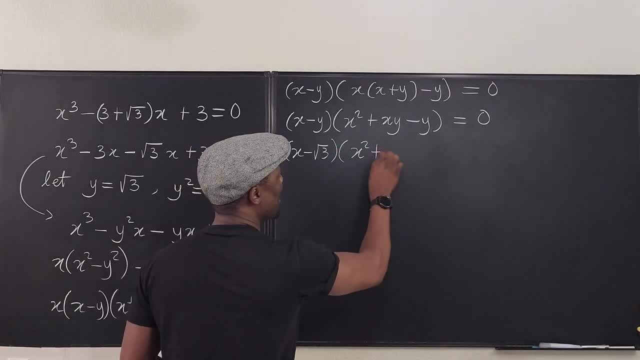 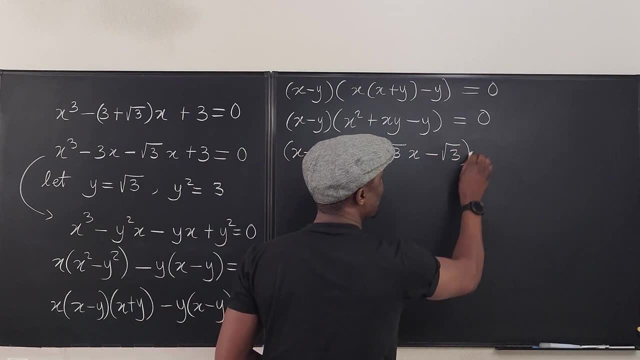 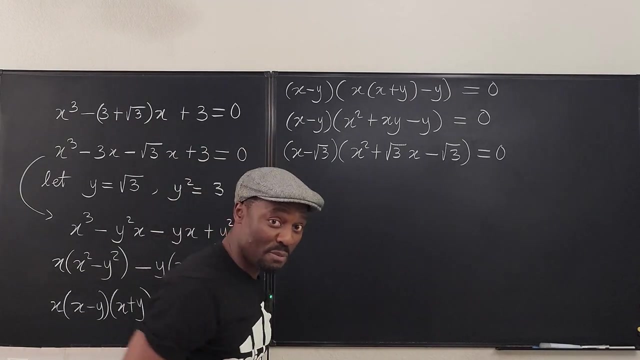 times x squared plus X times the square root of 3, which is the square root of 3 times X minus the square root of 3, is equal to 0 by the product. by the zero products rule, the product of two numbers can only be equal to 0 if one of them is. 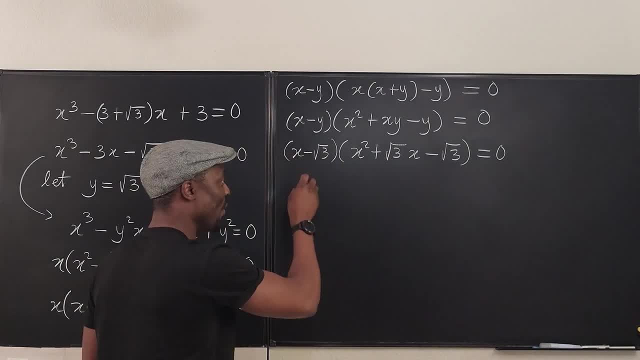 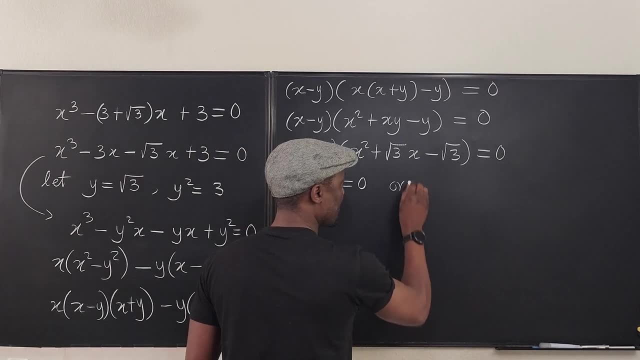 0 or both of them are zeros. so we know that X minus the square root of 3 is equal to 0, or x squared plus the square root of 3, X minus the square root of 3 is equal to 0. this gives us the first answer, right. 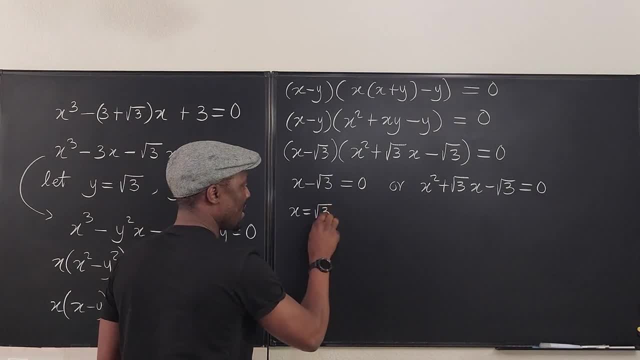 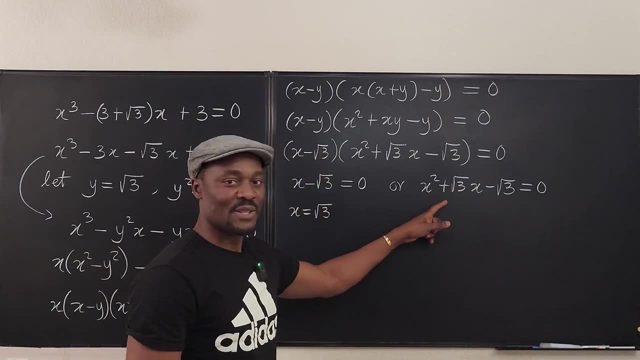 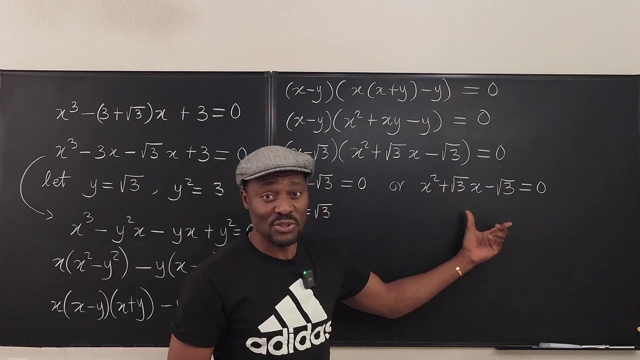 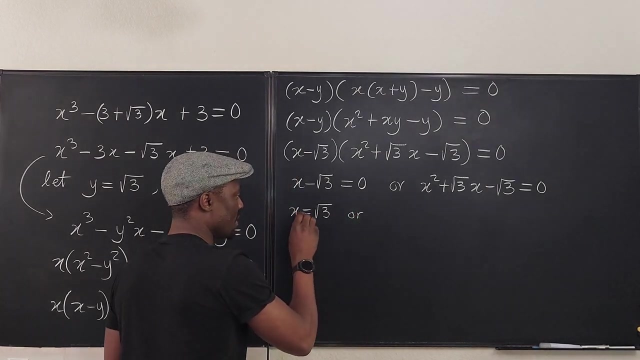 X is equal to the square root of 3. remember I told you at the beginning we have to get three answers. well, the two other answers are coming from this quadratic equation, even though it has radical, or what you call irrational coefficients. so what should we do? well, it's gonna be, or let's go this: X 1. 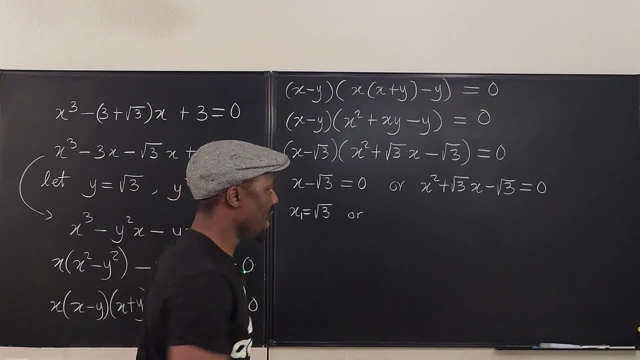 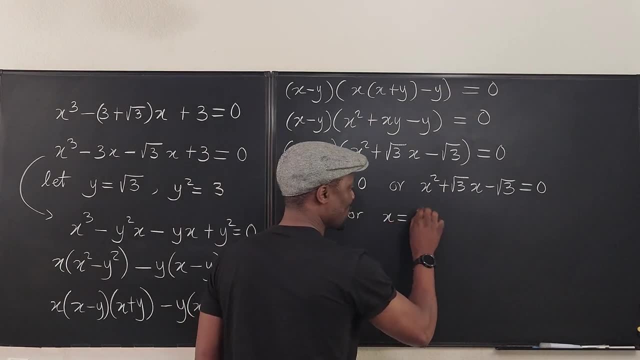 actually so. let's say: there's X 1, there's X 2, there's X 3. let's find X 2 and X 3, the quadratic formula here. So we know that x will be equal to, plus or minus, the square root of b. 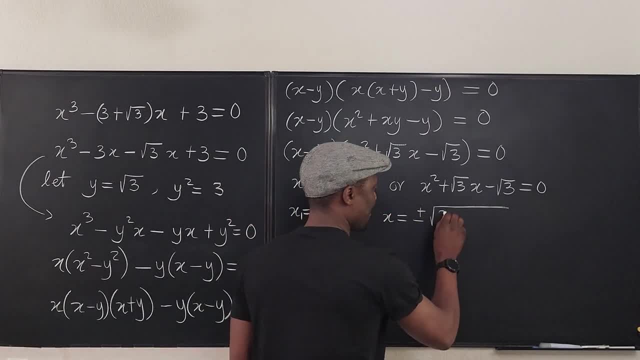 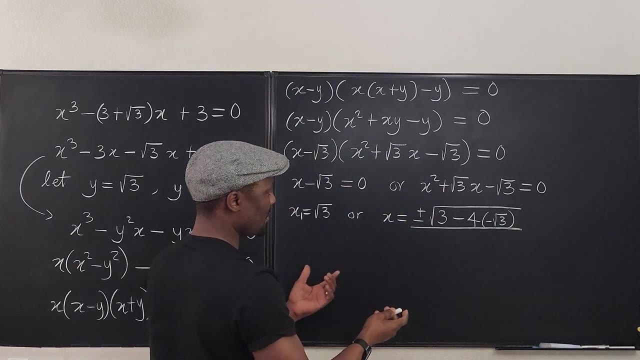 squared. What is b squared here? It's 3 minus 4ac. That's going to be 4 times 1 times c. What is c c is minus 3.. Minus, sorry, square root of 3.. Okay everything. Hey, something is wrong with. 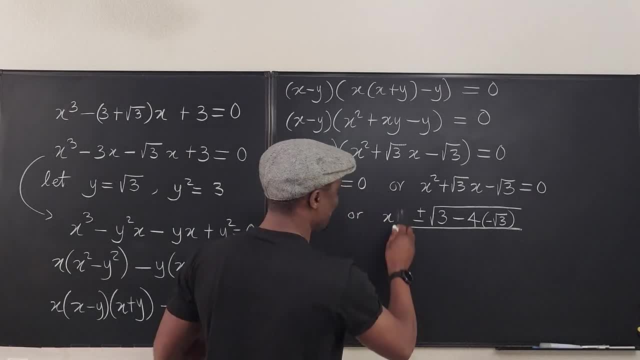 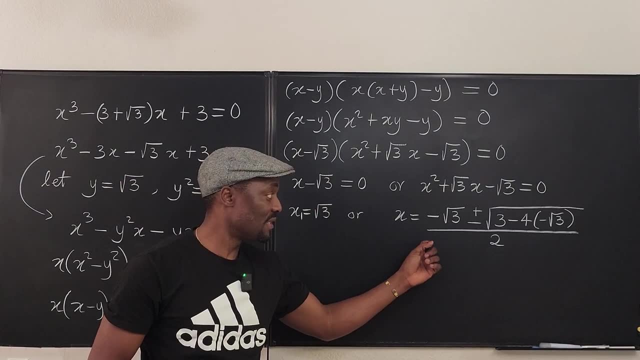 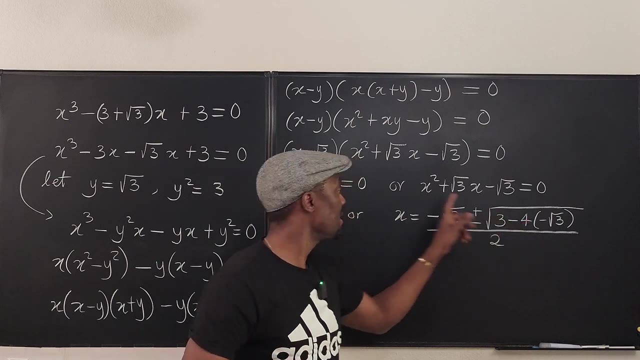 my formula: x equals minus b, Minus b equals minus b. And what is b? I have to rewrite this. So here it is rewritten and that's it. It's minus b, plus or minus square root of b squared minus 4ac. Our a is 1 here and this is our c, minus square root of 3, all over 2 times a: 2. 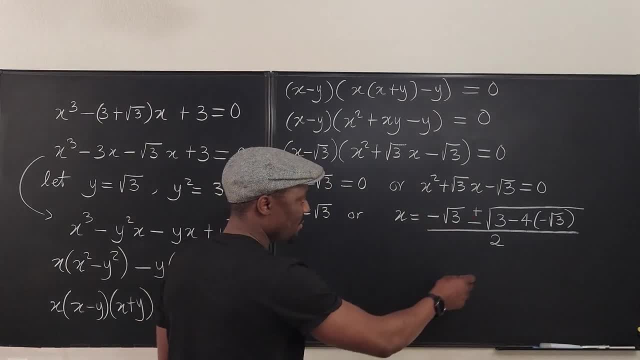 times a is just 1.. So we can say from here: if we clean this up, this is going to be 3 plus 4 rad 3.. That's what's going to be: 3 plus 4 rad 3.. That's what's going to be: 3 plus 4 rad 3.. That's. 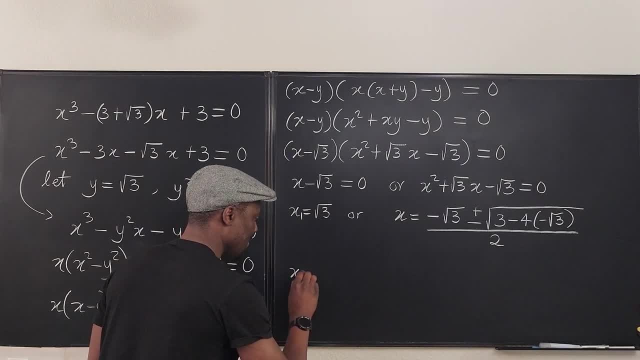 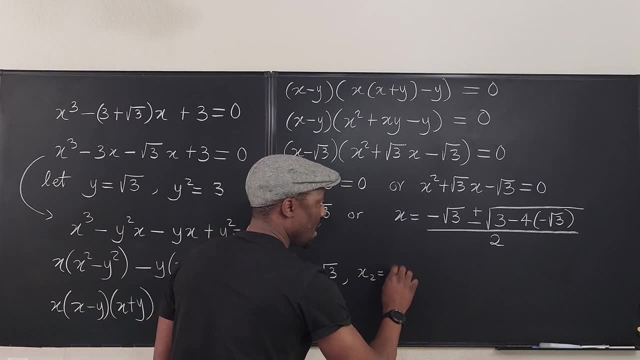 going to be up there. So we can say that x1 is equal to the square root of 3.. We can say that x2 equals just what it is here: negative square root of 3 plus the square root of 3 plus 4 root 3,. 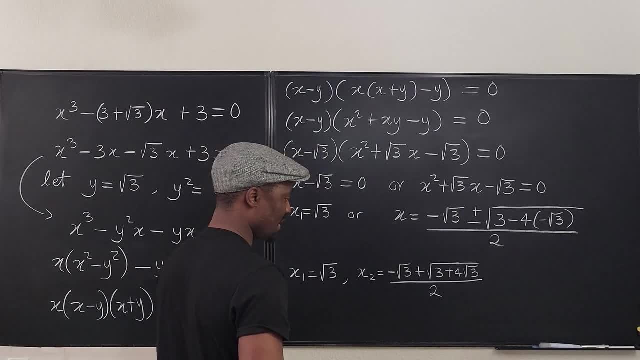 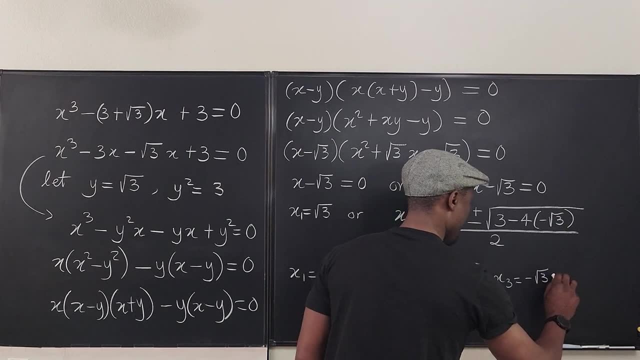 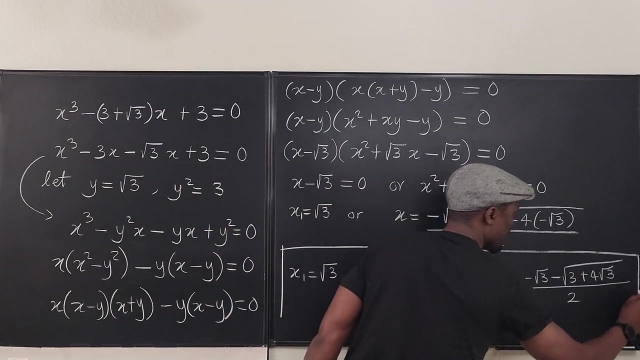 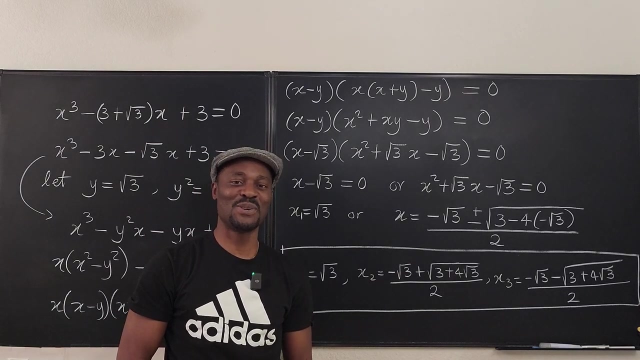 all over 2.. And our x3, is going to be negative: square root of 3 minus the square root of 3 plus 4, square root of 3, all over 2.. This is the solution to this problem: Never stop learning. Those who stop learning stop living. Bye-bye.